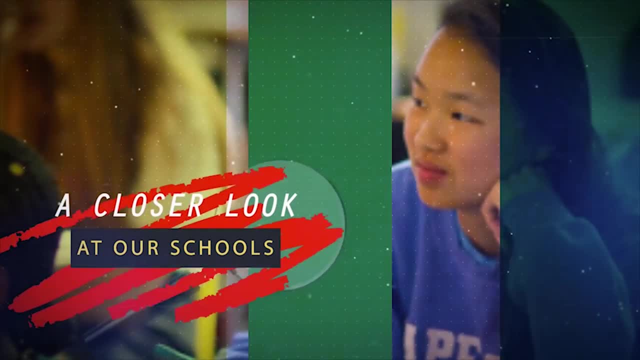 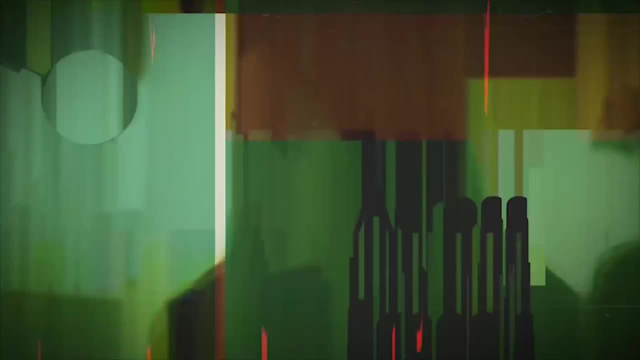 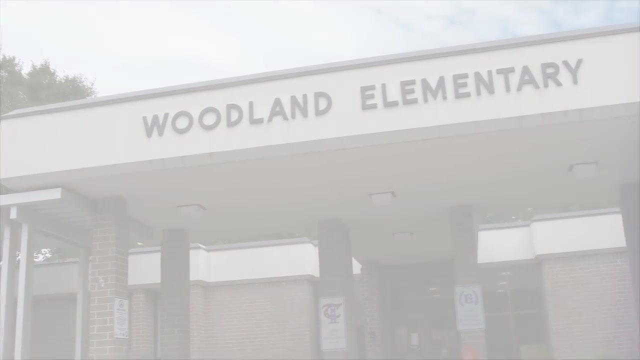 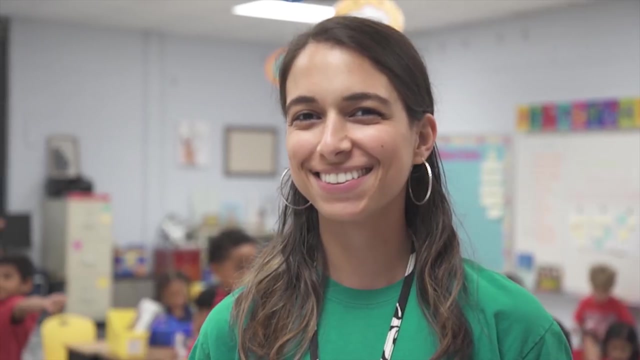 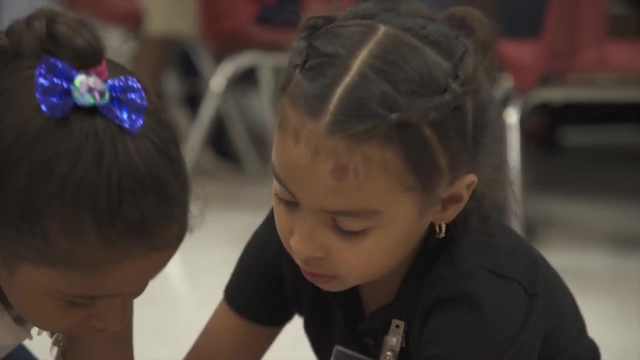 When people think of school, most people think of four walls. Here at Woodland, when we think of school, we think of the people: The students, the teachers, the parents, the community. It takes all of those members to make our school successful. We are a family that wants. 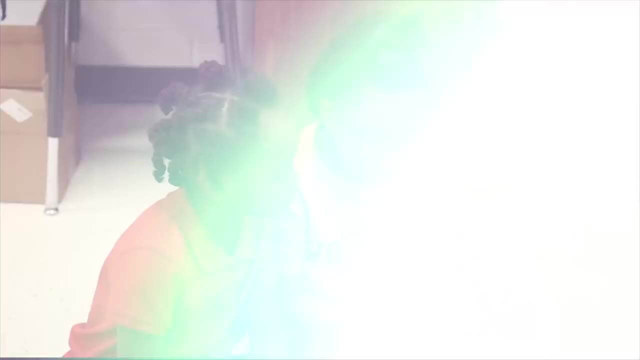 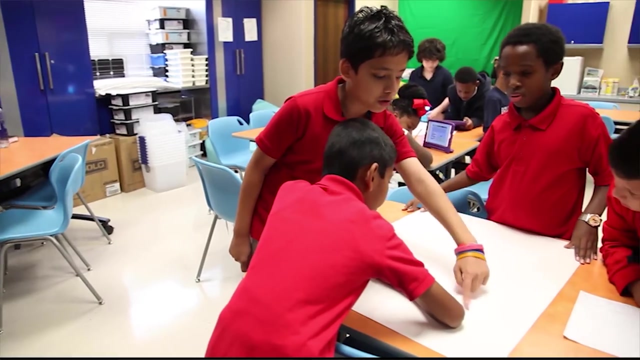 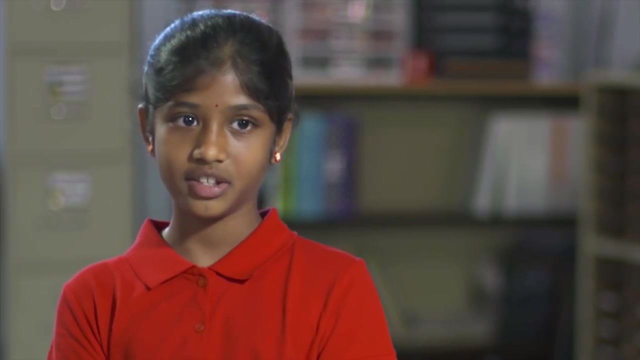 to see each and every student achieve success, High levels of learning for all of our kids. I think we breed excellence. We work really hard here and the kids work really hard here. Woodland is awesome and every single class, every single teacher is really great. 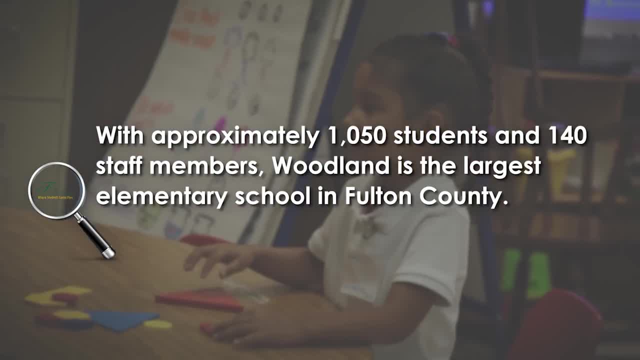 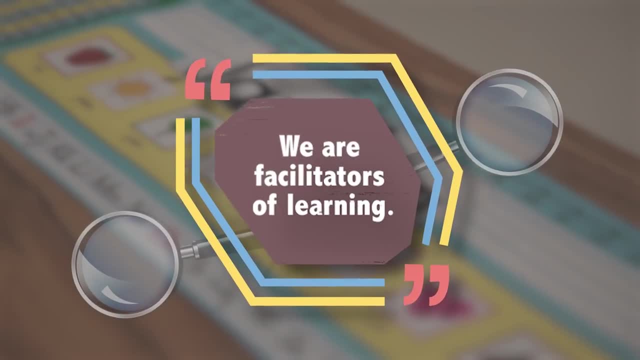 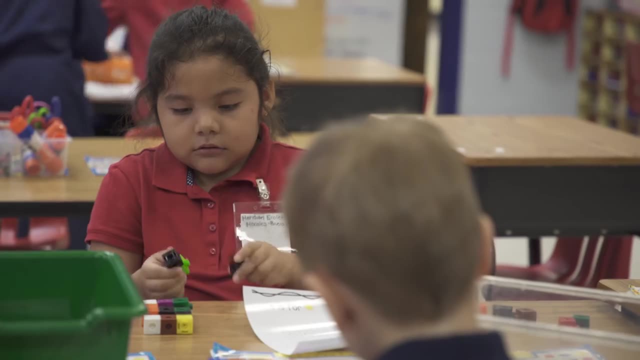 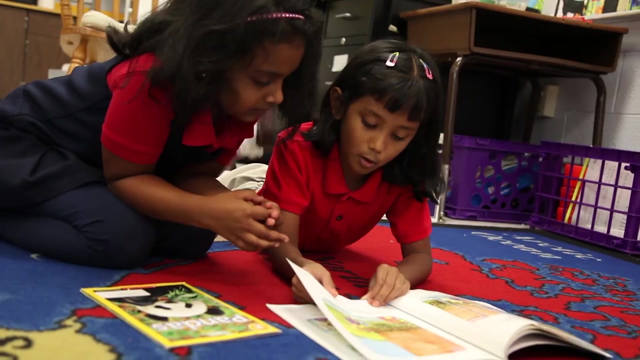 Well, we are facilitators of learning. So in the Woodland classroom you'll see teachers guiding students to become creative problem solvers. You'll see a lot of interaction among the students. You'll see guided reading groups. You'll see a lot of. 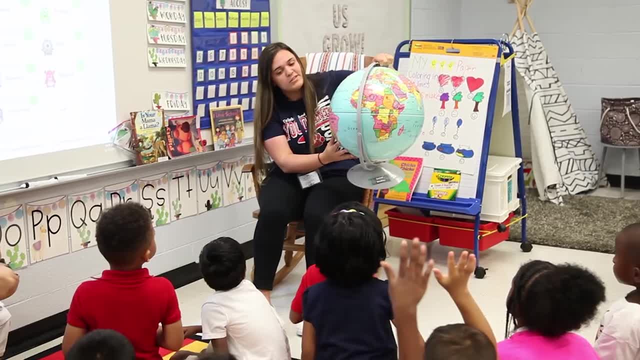 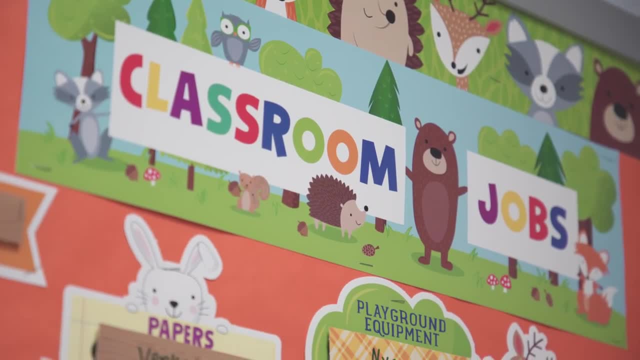 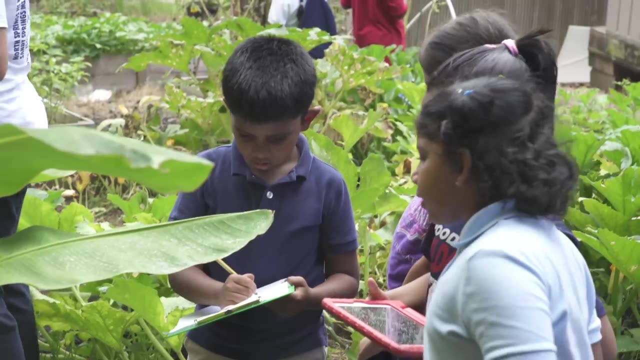 hands-on activities. The teachers, they're nice, They like listen to what you're saying, They don't just ignore you. We offer a lot. I mean we have after-school programs, We have Lego, WeDo, We have robotics. 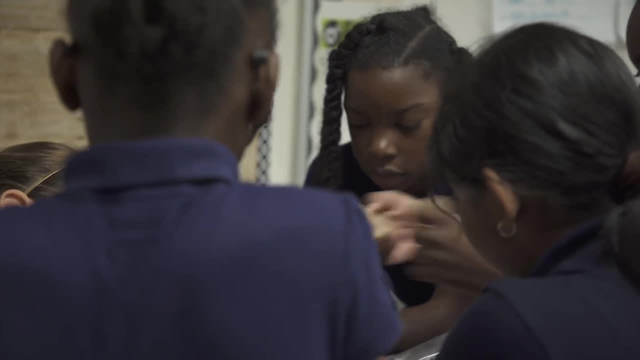 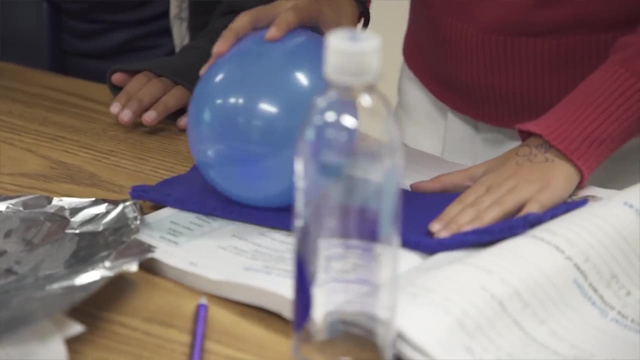 We have Science Olympiad, We have chess, We also have gardening, where the kids work in the gardens And then they actually take the food that they get in the gardens and they end up baking with it. Well, we're a state-certified STEM school, which is really amazing, So we don't just 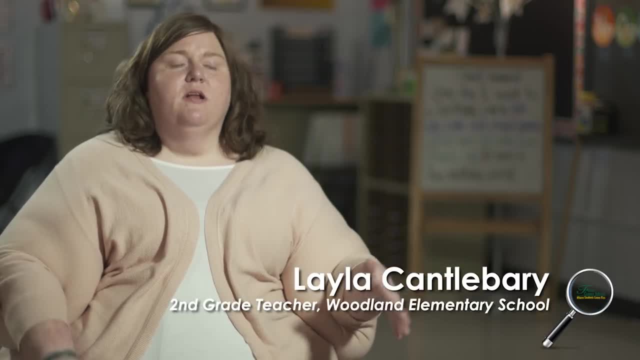 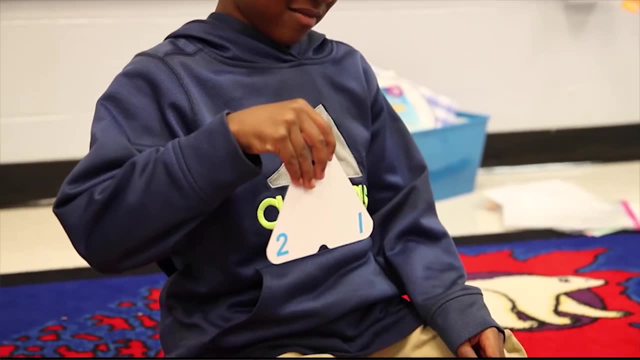 teach our science and our math silos separately, but instead we integrate that into our whole curriculum. We use the engineering design process, the EEP, throughout the day. We don't just use it for science. The aquaponics lab is like the coolest place in the school, Like all the kids love to. 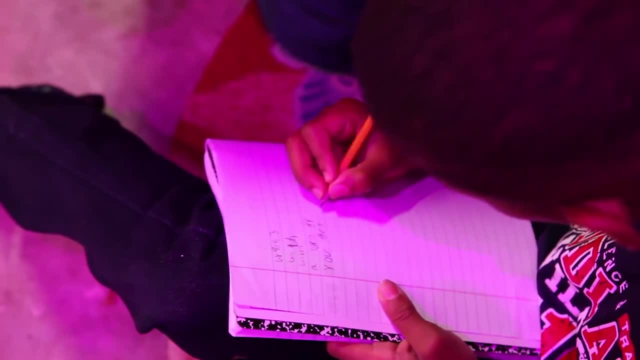 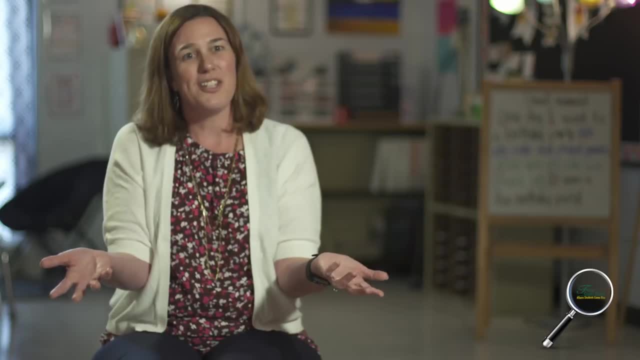 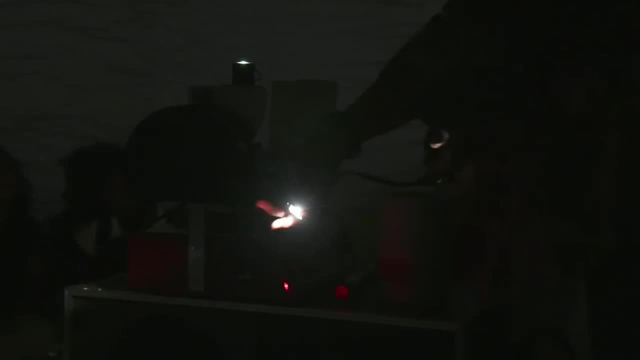 And they learn like just a lot of math And we immediately start doing math and science. They'll take the fish out, they'll weigh the fish and, you know, measure the fish to see how much it's growing. Starr Lab: we have students go in there and they not only do learn about the stars and 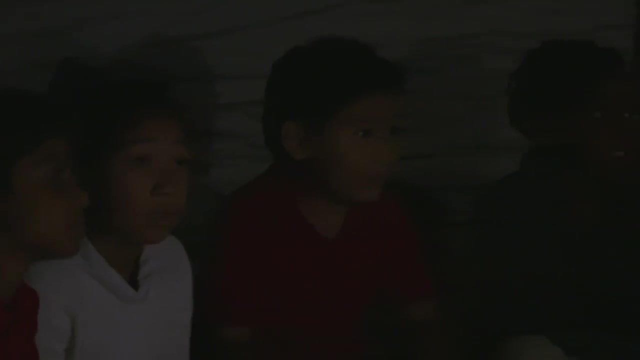 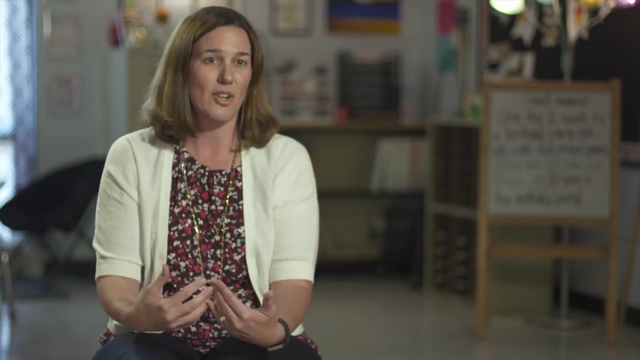 the constellations, but they, like Miss Mason, integrates, like for second grade. for example, they learn about native Americans in Georgia, so she does a lesson about that with them in the Starr Lab. So we have all sorts of creative learning, like woodland, things outside the box, like 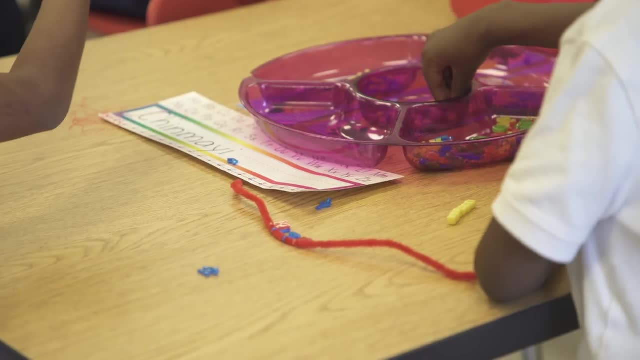 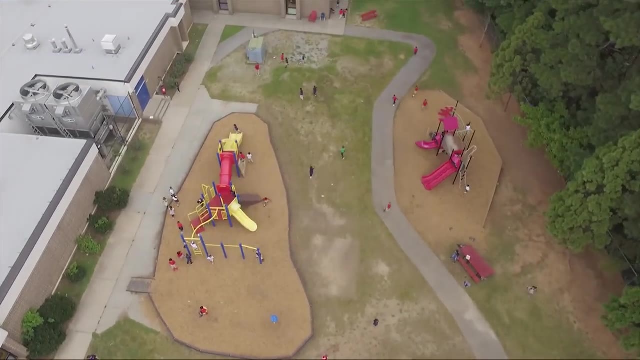 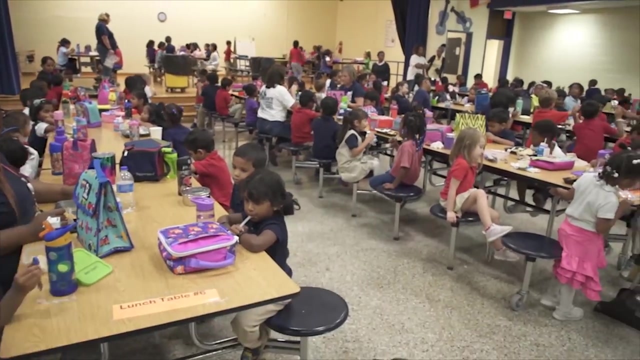 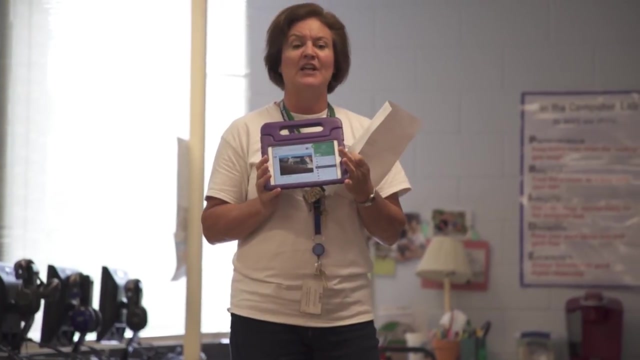 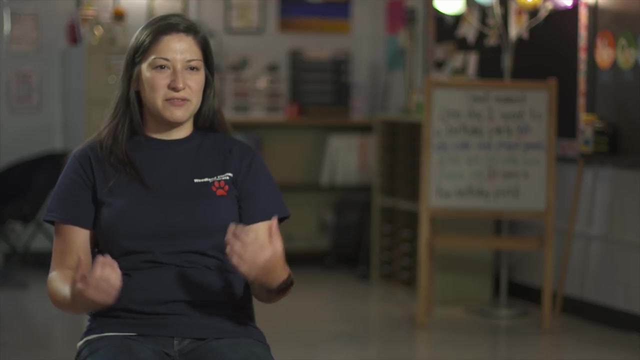 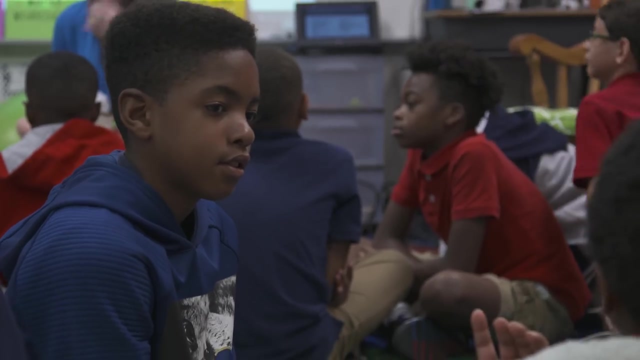 this is the box And we're doing this right here. The teachers have really worked to create community and create kind of a family feeling within their classrooms. We have pride time first thing in the morning where the teachers talk to their students about different character traits, discipline or integrity or excellence. 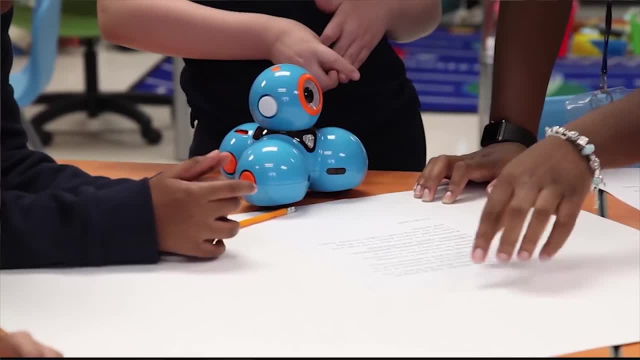 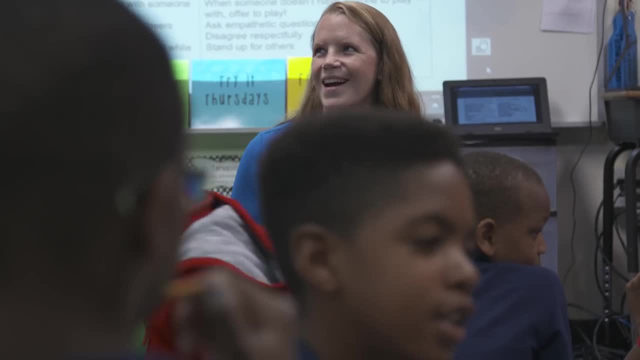 We are a community-based school. We get to know each other. We do a lot of different things with our PBIS team, which is, you know, they seek out ways to increase our- you know- positive culture in our school and bring people together as 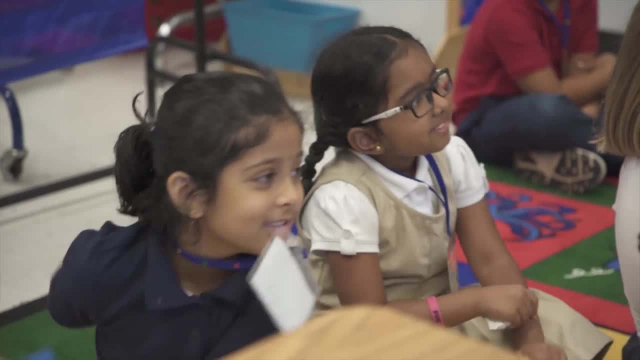 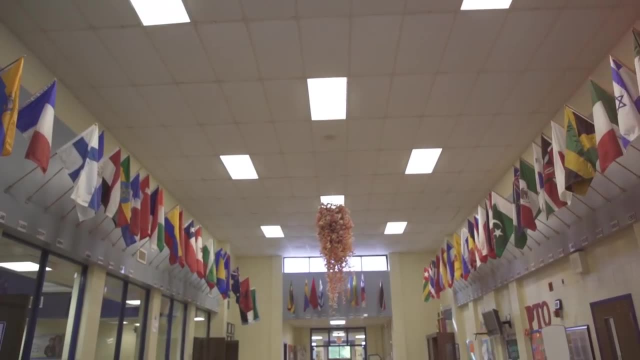 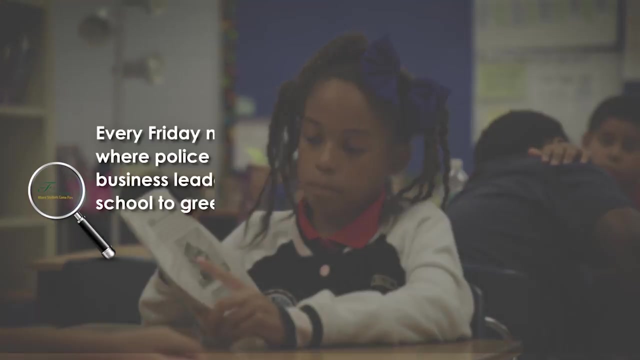 family members, just to get to know one another. We have a diverse population, which represents the city of Sandy Springs, and we celebrate that diversity. I'm sure you've seen the flags that fly over our atrium. Each of those flags represents the cultures that are here at Woodland. 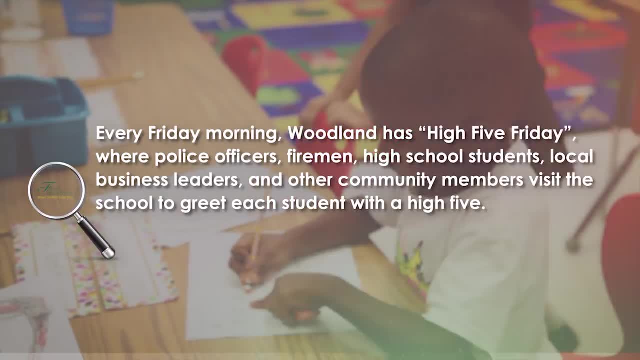 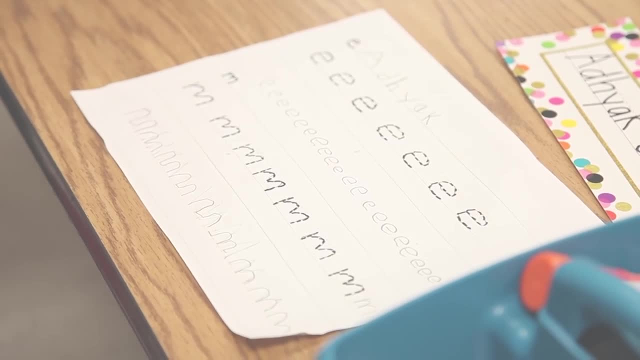 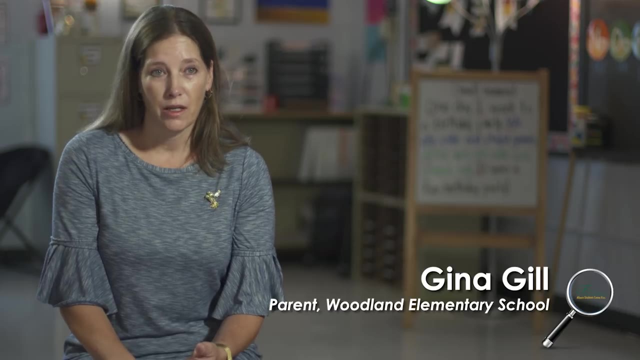 Parents get involved in a lot of different ways. We have parents that will take materials home to sort for teachers. We have parents that will help with PR with the website. We've got a parent that just does the information online for the marquee. 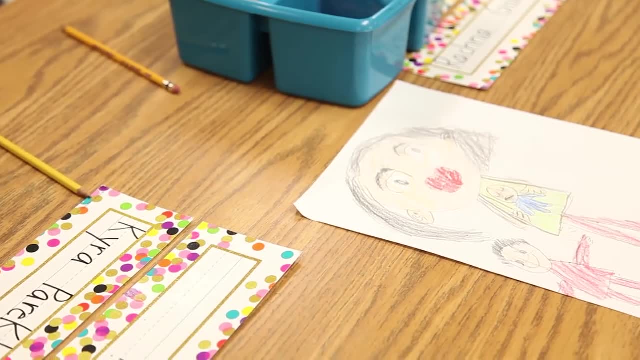 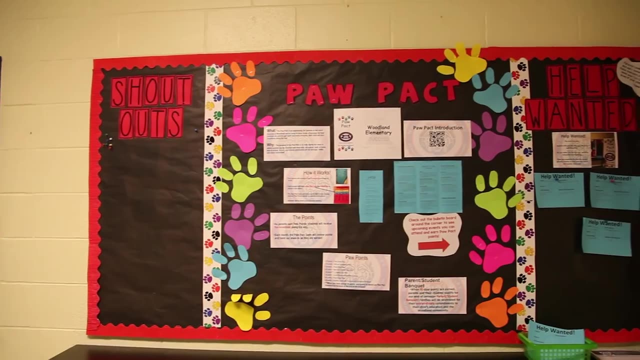 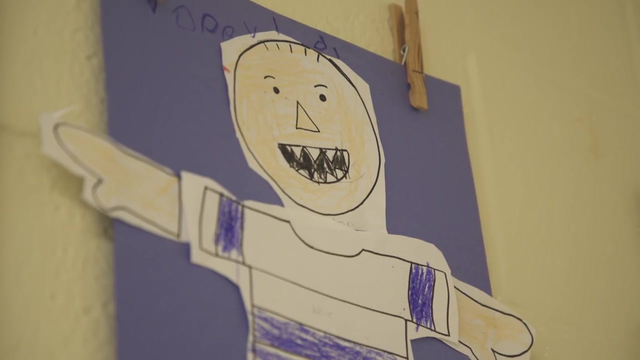 We have parents who give and have matching corporate contributions. Our design thinking team ended up creating something called a Paw Pact, and a Paw Pact is where parents come in and they volunteer, they do different activities and they get these points for their kids to do: free dress and things like that.